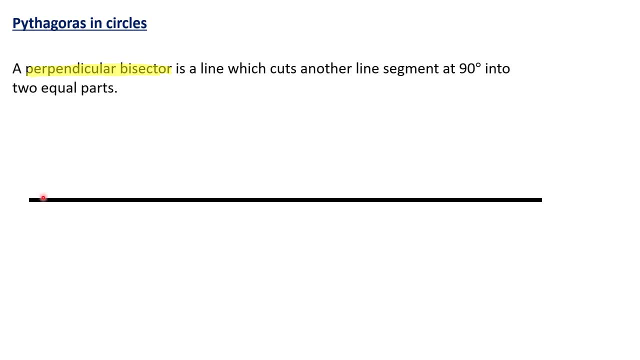 This black line here, This one here. So a perpendicular bisector is a line that's going to cut that line in half at right angles. So say, for example: say, if I find a halfway point, it might be like somewhere here: See, this line, That is not a perpendicular bisector. 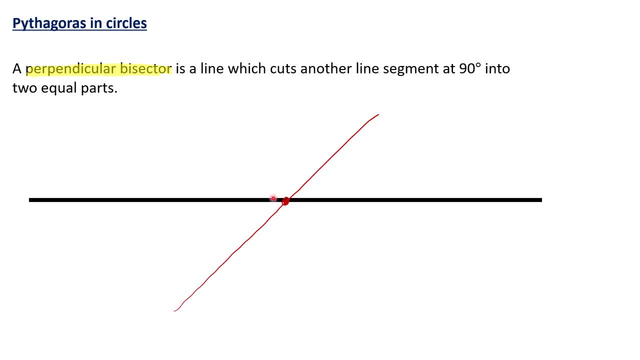 because it does not cut it at right angles here, here, here and here. Okay, so I'm just going to rub that out. So if I get my halfway, halfway point there roughly, So this dashed line I'm doing and blue here, This line, here is what we would call the perpendicular. 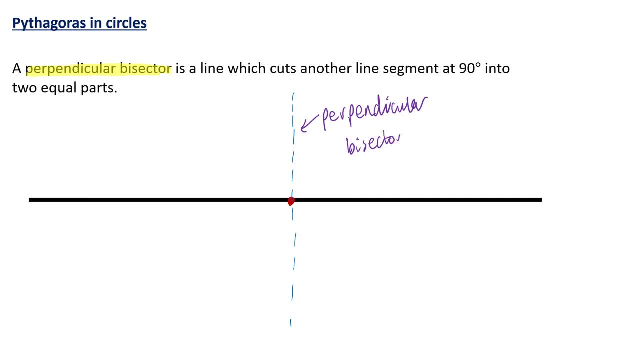 bisector, because it's cut the line in half. It's cut it at right angles and that's important because we can use Pythagoras in right angles, And that's important because we can use Pythagoras in right angles, triangle, triangles. so if we knew that this line, if we knew that the full line was 50 centimeters, 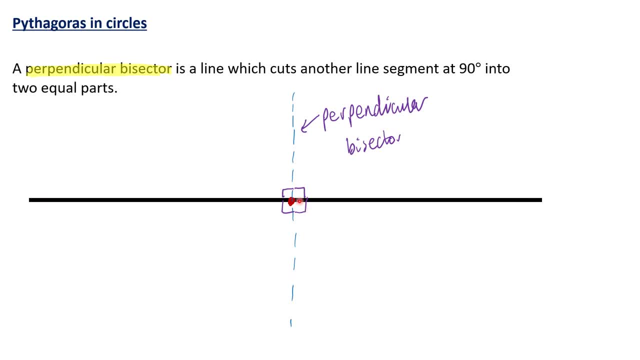 well then, because we've got this perpendicular bisector, we then know that this bit here is 25 and this bit here is 25. okay, let's see how we can use this, but before we do that, we need to look at one more thing. when we look at circles, there is some information you need to know you. 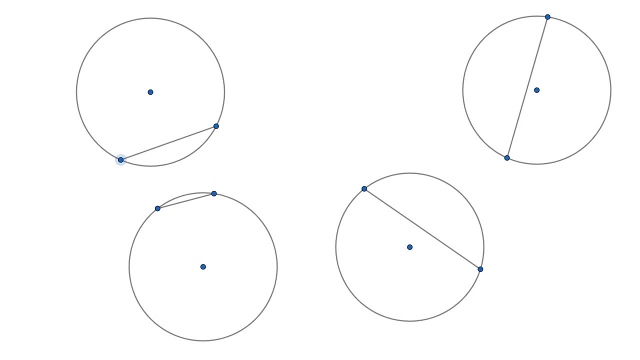 need to know what the radius is, what the diameter is and what the circumference is. circumference is distance from the outside. the radius is from the circumference to the center. diameter is from one point in the circumference through the center to the other. but here, if we have a look, these lines, 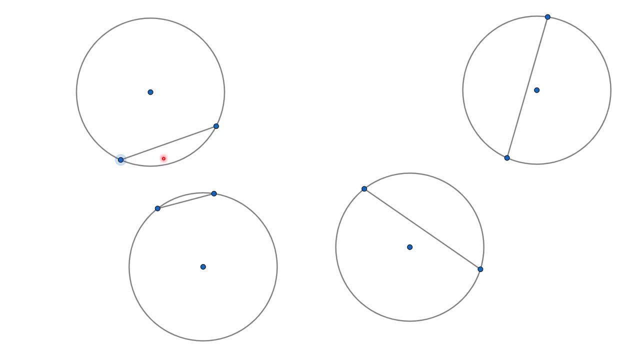 here. that's not the circumference, that's not going around the edge, it's not a radius, because it's not going into the center, and it's not a diameter. diameter needs to pass through the center and you can see that in all of these triangles here, the line that i have drawn does not pass through. 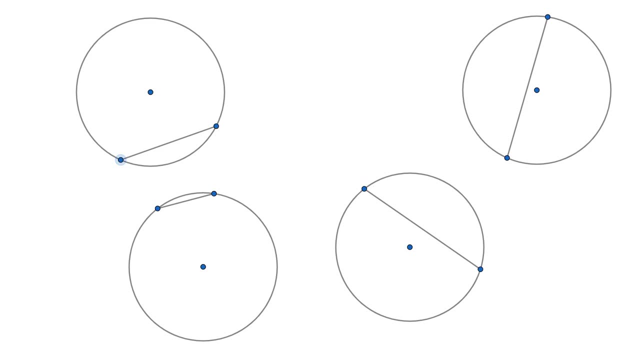 the center or touch the center. therefore it is not a radius or a diameter. these lines here are known as chords. okay, and often exam questions with Pythagorean circles. look at chords. but this isn't particularly interesting so far. but when it becomes interesting is when we draw a radius from the center through. 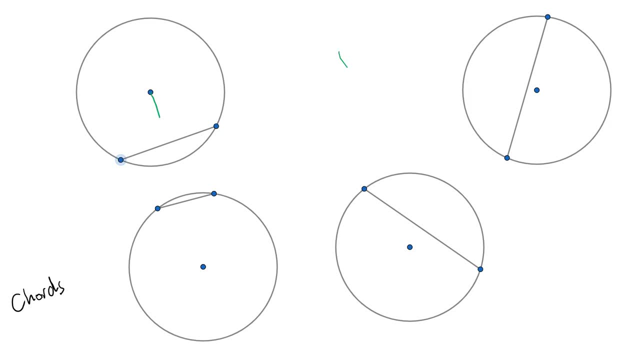 that chord. so see if i were to draw the radius from here to here. the thing that's really nice is see that chord. that green line that I've just drawn creates a perpendicular bisector to the chord. okay, so the radius cuts a chord in half, into two equal parts. so if I were, 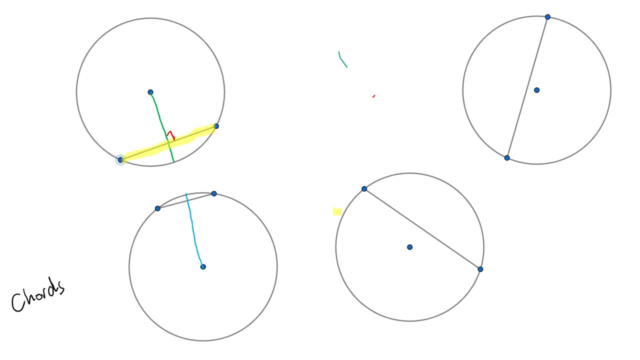 to draw another radius here, then I've got right angles and I've cut that chord in half. if I draw in a line, my radius here, that green line, goes from the centre to the circumference, then I've cut that chord in half at right angles. similarly here, if I draw a chord that 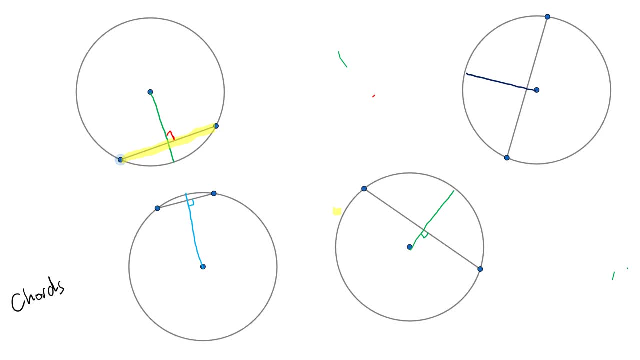 chord if I draw a radius. sorry, that chord has been cut in half at right angles, so a radius acts as a perpendicular bisector to a chord. okay, we can use this fact now to try and now use this information to try and work out some things in Pythagoras within circles. 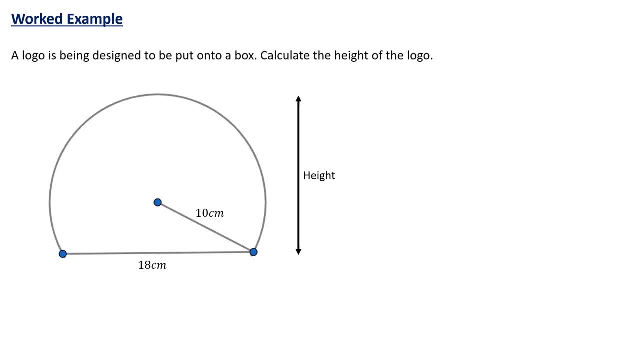 okay. so here we've got a worked example. this is a very kind of examy style question. a logo is being designed to be put onto a box. calculate the height of the logo, okay? so let's have a look at the information that we've got here. we've 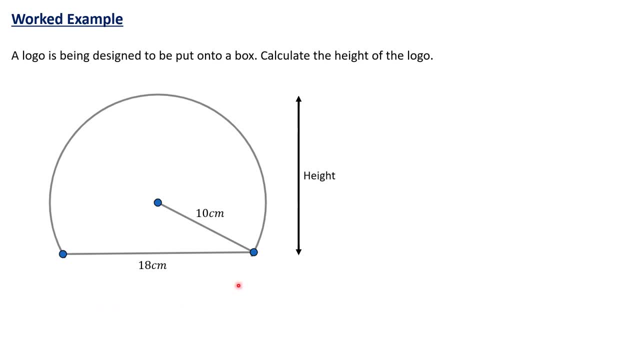 got part of a circle. okay, I've got part of a circle here. we don't have the full circle. if it was a full circle, we would have this little part in here. what other information do we have? well, we know here that we've got from the centre, we've got a point here from. 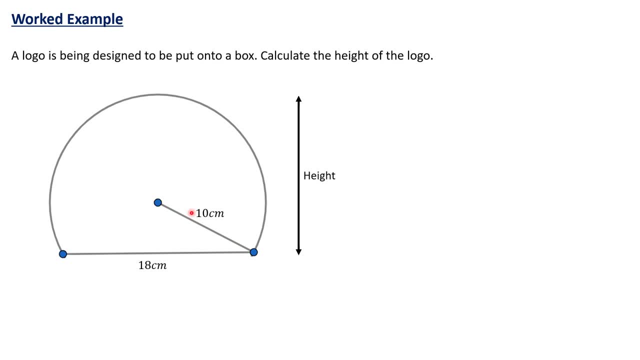 the centre to the circumference. so see, because I've got the centre to the circumference, I know that this 10 centimeters here is the radius. okay, that is the radius of the circle. so if the radius from there to there is 10, that means that from there to there is 10, and there to there and there. 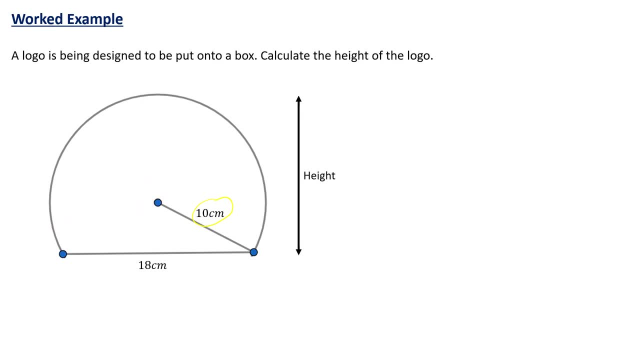 to there and there to there. I'm going to draw a line in here, from here to here. the length is not 10.. okay, it's not 10 because this is not the edge of the circle. if the circle was extended all the way around like so and my line went to here to there, that length would be 10. okay. 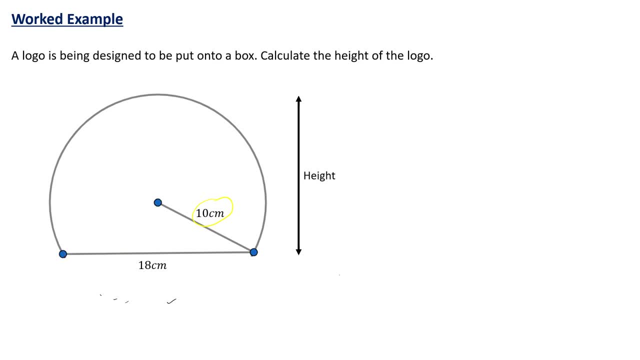 but in our diagram we do not have that. I'll just rub that out there. so what we know so far is that the radius is 10.. so if we have a look at what we want to work out, we want to work out the height of the 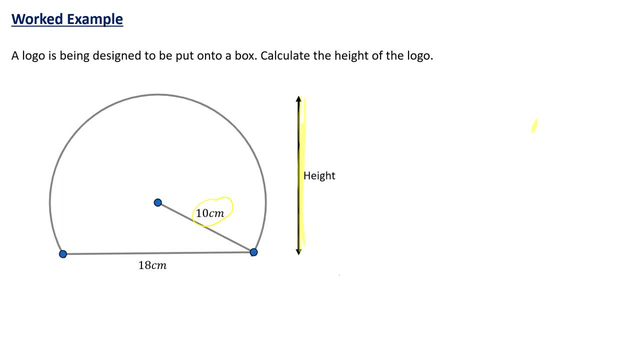 circle. let's try the height of this logo so see if we know. if we know that the radius is 10, that means that we know that from this point here to this point here, from there to there, that's a radius. so I know that from there to there is 10. so I'm going to mark. 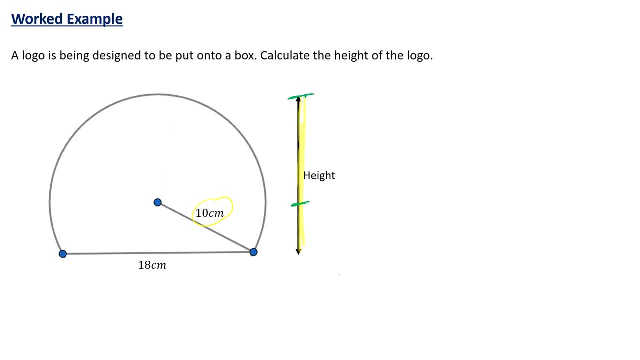 that on at the side. I know that from there to there is 10 centimeters. so to work out the height, I'm going to need to work out this little bit from here to here. do you see that? okay, so what can we do? well, we've got a cord at the bottom here. here's. 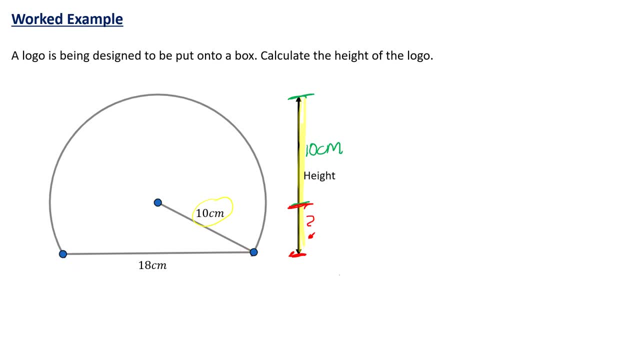 our cord. what we can do is we can chop that in half. see, if we draw a line down from our radius, that's going to create a perpendicular bisector. okay, we always want to try and form a right angle triangle, and we've done so here. so what we can do is we can do some maths. 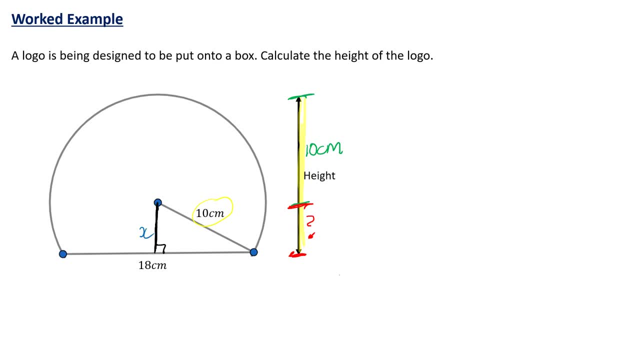 and we can work out that value there, which we'll call x. okay, what I'm going to do is I'm just going to draw this triangle again at the right of our page. this time I'm just drawing the right angle triangle. okay, so the radius was 10 centimeters. this distance here would be nine, because, remember, 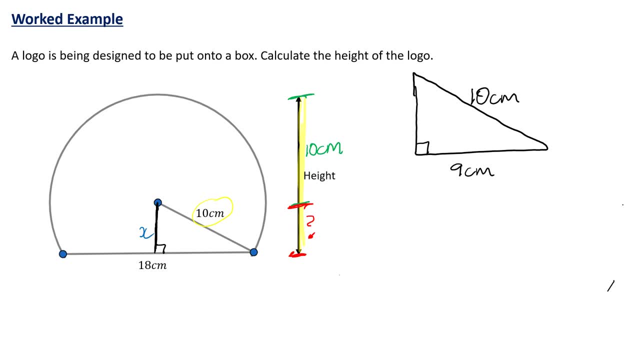 it's a perpendicular bisector. it's chopped that in half and we want to work out x. okay, so we're using Python as a big theorem here and you can hopefully see that we're wanting to find a smaller side. so we're going to be subtracting: x squared is going to be 10 squared minus 9 squared. 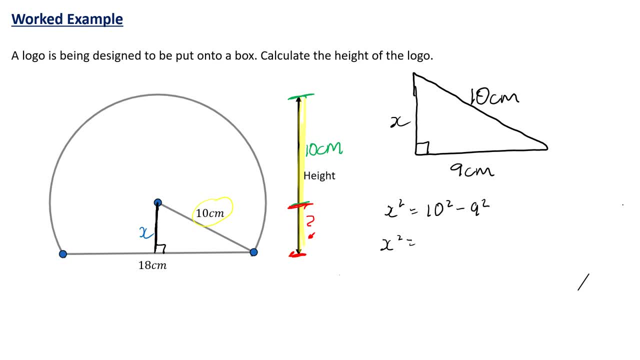 x squared equals- I'll just do this on the calculator- 10 squared minus 9 squared. so x squared is 19. so x is going to be the square root of 19. that's going to be 4 point something: 4.4 to 1. 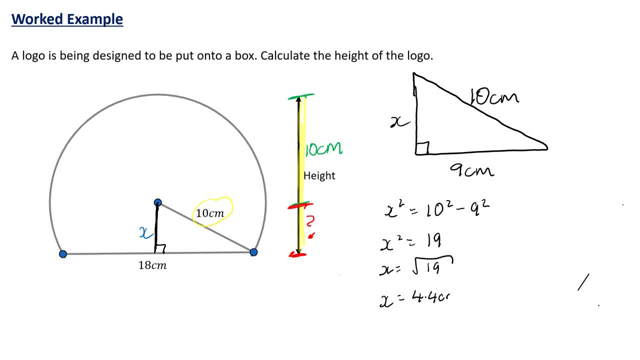 decimal place. okay, so what we just found out is that this length here is 4.4. from here to here is 4.4. that means that from here to here is 4.4. so if I want to work out the height of the 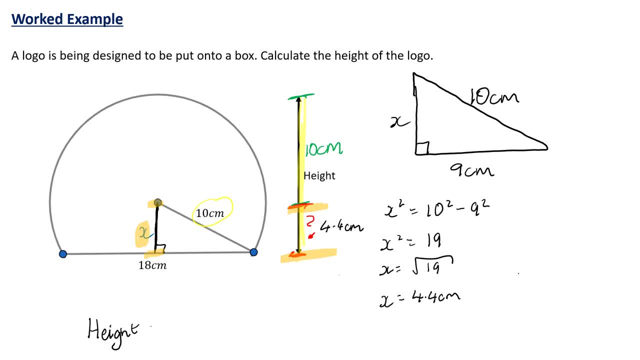 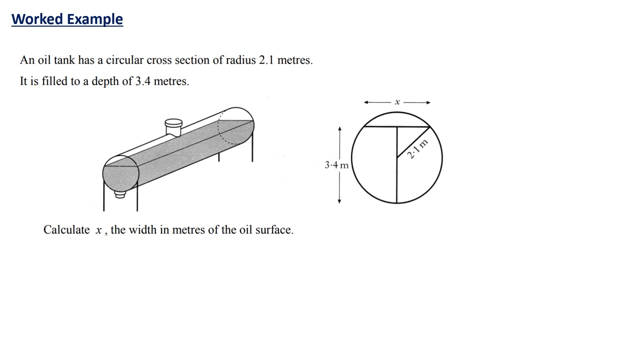 logo, the height is going to be 4.4 plus 10 centimetres, so the height of the logo is 14.4 centimetres. okay, we've got one more past exam question to show you as a worked example. okay, example two: an oil tanker has a circular cross section of radius 2.1 metres, so without 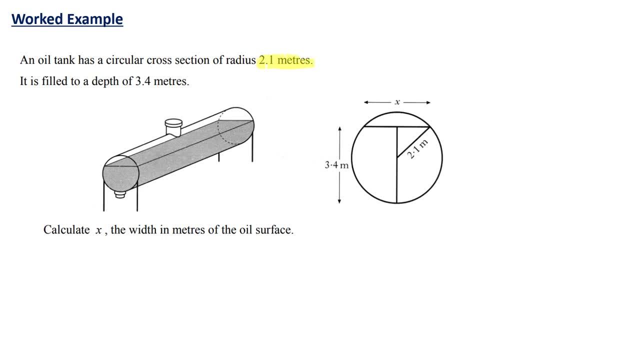 even looking at the question, we've been given the radius. that's quite nice. it is filled to a depth of 3.4 metres. calculate x the width in metres of the oil surface. okay, so let's have a look at this diagram. what information are we told? so we're told the radius. we are told that from here to here. 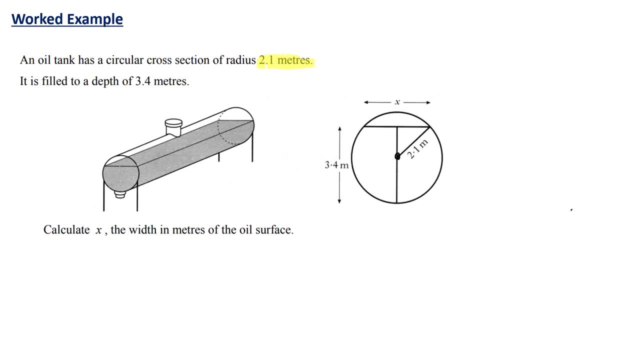 is 2.1. i'm just going to mark that centre on a bit clearer. there's the centre, so from the centre to the circumference, to a point of circumference, is 2.1, and we've got this line on in here so i can do this little right angle okay. so it looks like what we're going to do is we're going to need to. 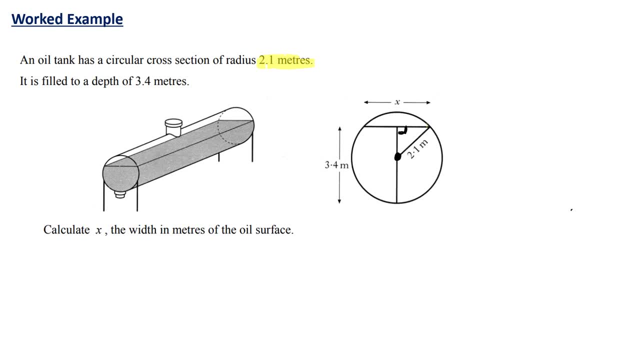 work out. if i highlight this, we're going to need to work out this little bit here and then, once we need to work out this little bit here, and then, once we need to work out this little bit here, on that, we can then double it to work out the value of x. so i'm going to draw this triangle. 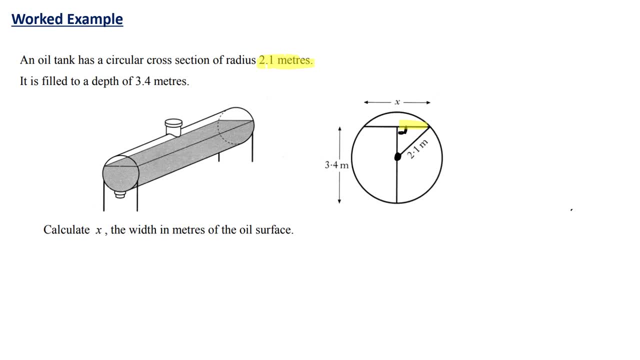 again at the side. i'll do it here. okay, so i've got my radius being 2.1 metres, but what is okay? the green pen here, the black, sorry, what is that bit? what is the length from here to here? okay, so we need to go back to our definition of what a. 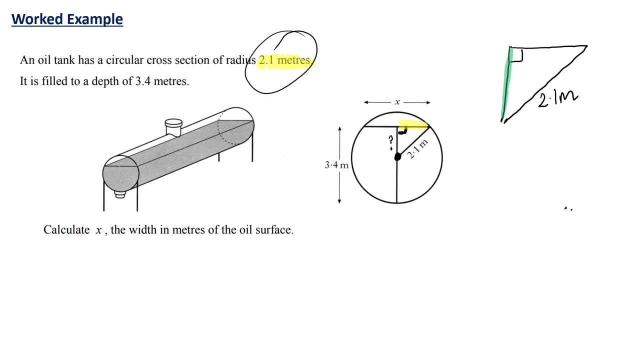 radius is radius, if you recall, goes from the centre to the circumference. okay, so c here on a diagram. if i just go in red c from the centre to the circumference, i know that from there to there is 2.1 metres. okay, if from there to there is 2.1 metres, and from here to here, 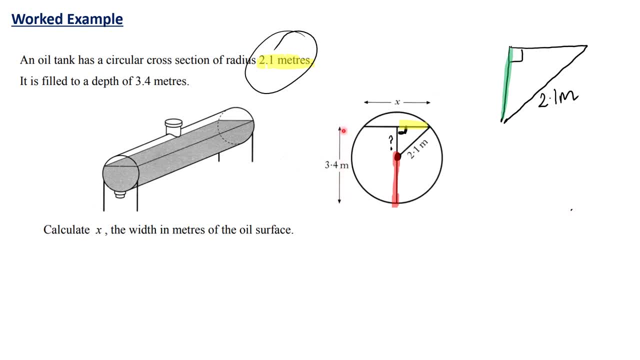 there we go from here to here is 3.4 metres. we'll see to work out this little bit up here to work out like the value of the question mark, i can do 3.4 subtract the 2.1 from the radius. okay, i'll just do that there. so that's going to be 3.4 subtract 2.1. 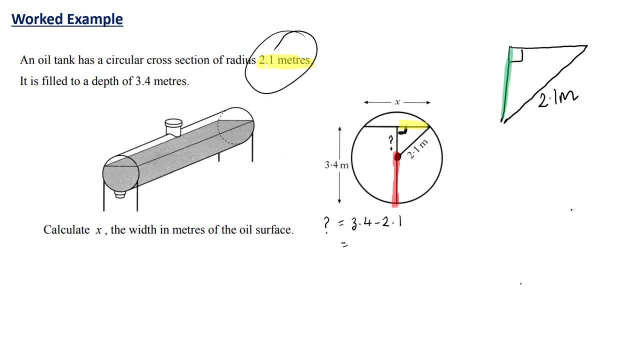 okay, 3.4 subtract 2.1, and that's going to be 1.3. okay, so now we've worked out that this value up here is 1.3 metres. okay, so what we can do now is we can now work out this value up here. i'm going to call it y. 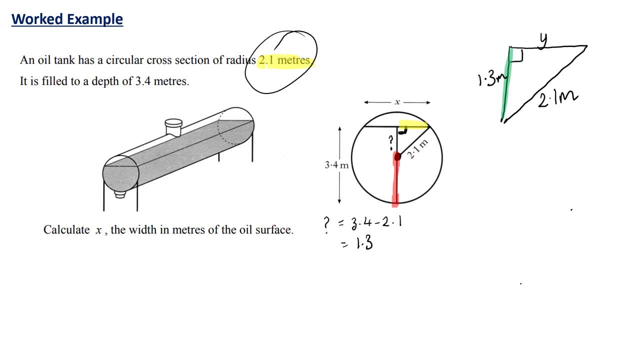 i'm not going to call it x, because we're looking for x in the question. so we're looking for a smaller side, so we're expecting that answer to be less than 2.1. so we're going to be using x. y squared is going to be 2.1 squared minus 1.3 squared. 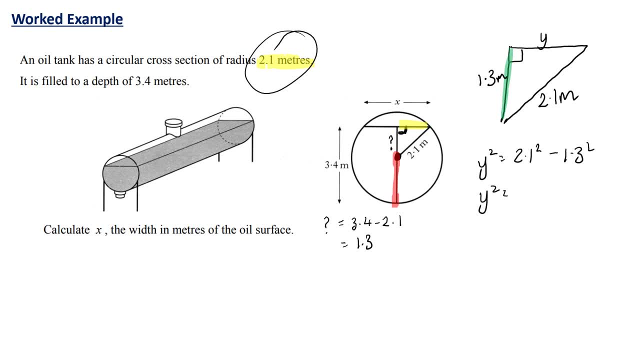 y squared. oops, just do this in the calculator: 2.1 squared minus 1.3 squared, that's just 2.72, and if we square root that, we get 1.6 to 1.. okay, so we want to work out the width x. that's a bit wee, dot dot dot. that just means therefore. 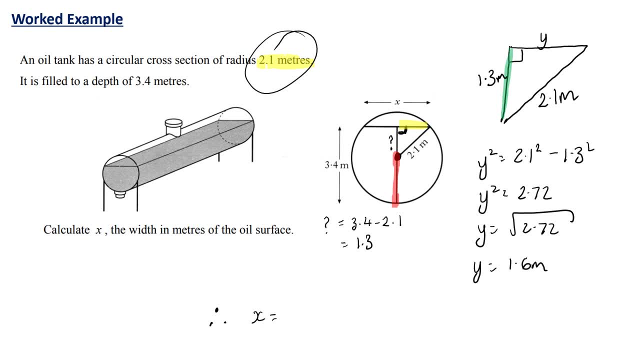 x equals. so we've just worked out that this length from here to here is 1.6. that also means that from there to there is going to be 1.6. so x is two lots of 1.6, which is 3.2 metres. 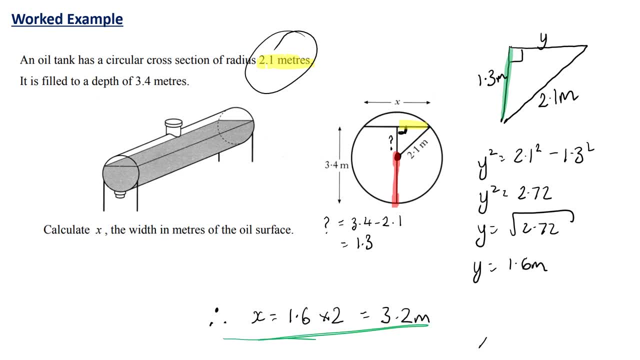 okay, so notice this goes up to 1.6. so that's going to be 1.6. okay, so notice this goes up to 1.6. okay, so notice this goes up to 1.6. so notice this question worked through a little bit differently from the last time.